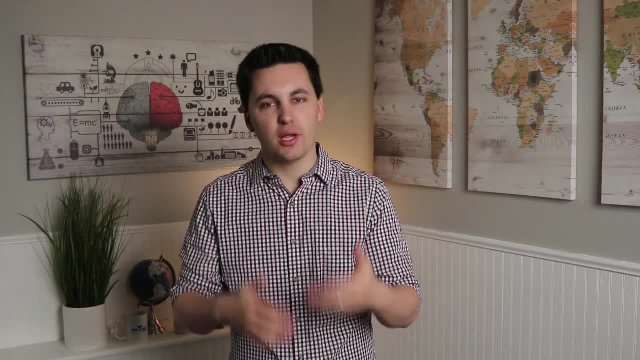 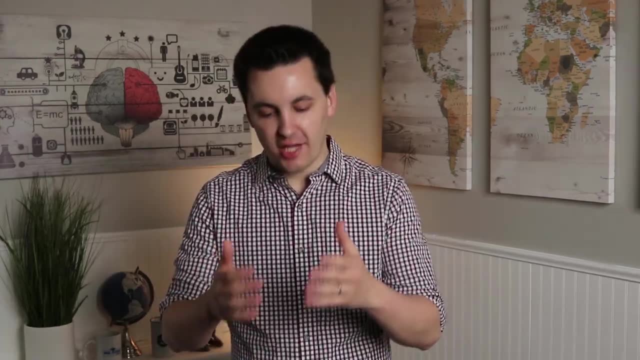 stay stable over time. This just means that our scores should not fluctuate that much if we keep taking the test. Our intelligence is not constantly changing every minute, and the test should reflect that. In order to check a test's reliability, researchers will test individuals multiple times. 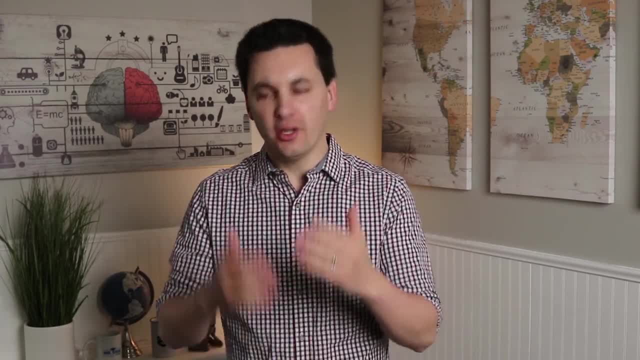 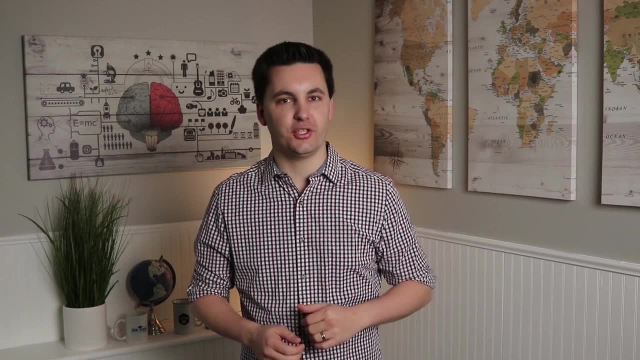 and may use the split-in-half method, which is when they split the test in half to see if test takers do better on one part of the test compared to the other part. Ideally, there should be a high correlation between the two parts of the test, which would show that the test is correlated. 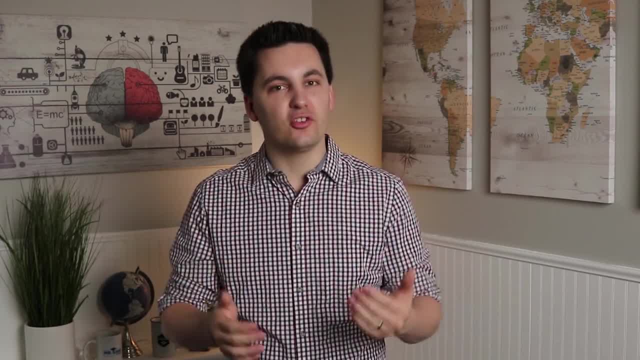 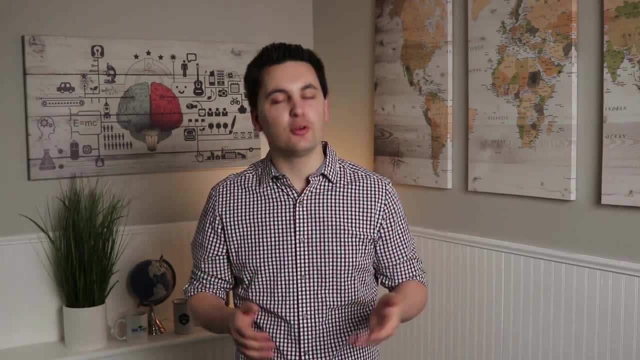 with itself. Lastly, the test needs to have validity. This just means the test is assessing what it claims to assess. Remember we talked about reliability and validity back in our Unit 1, Topic 4 video. We can break validity down into four. 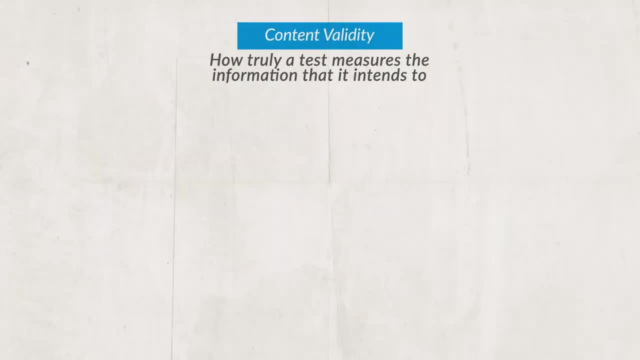 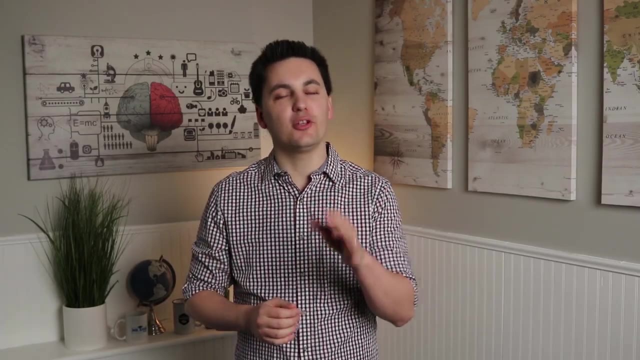 different types of validity. The first is content validity, which is to the extent in which a test inquires about the information or behaviors that are of interest. For example, a safety test at work is meant to assess you on different situations you'll experience while at your job. This test 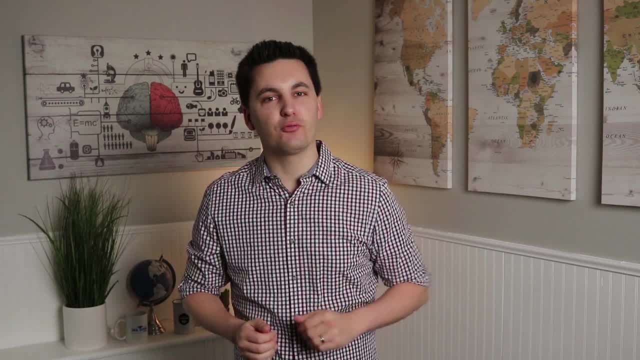 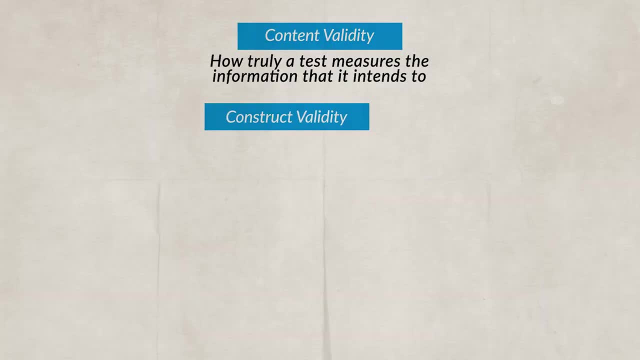 only has content validity because it's assessing you in the tasks that you'll be confronted with while working. If it asks questions about situations that you would not experience while at work, then it lacks content validity. There's also construct validity, which is to the degree in which a test can actually measure a specific trait or concept. 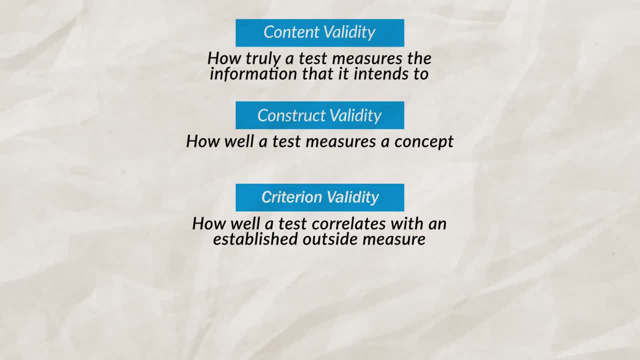 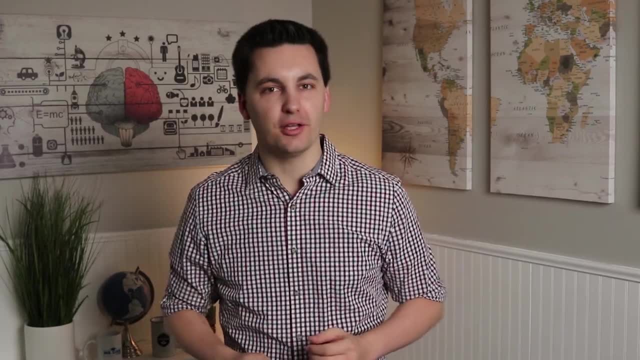 Criterion validity, on the other hand, checks to see if the test correlates with any outside variables or measures. This validity shows us how well the test correlates with a standard comparison. If it's low, the test may not be valid. Lastly, there is predictive validity. 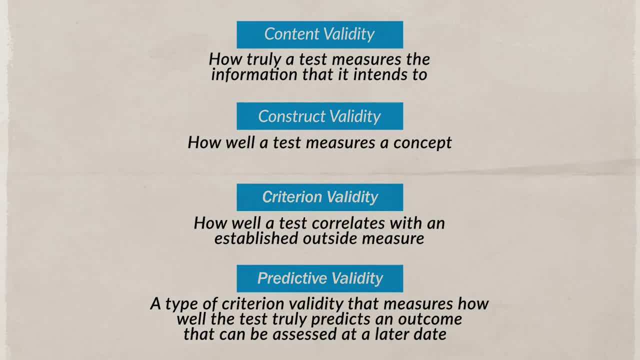 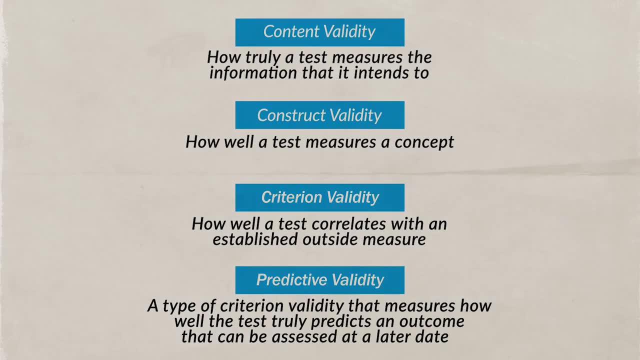 which predicts future performance. This validity can only be used when we have a large data set and is only useful at predicting trends and patterns. Individual tests and standardized tests do not have predictive validity for individual test takers. When looking at the results of intelligence tests, we can see scores from a bell curve. 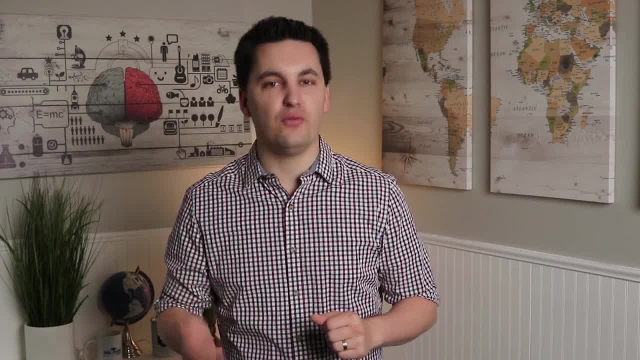 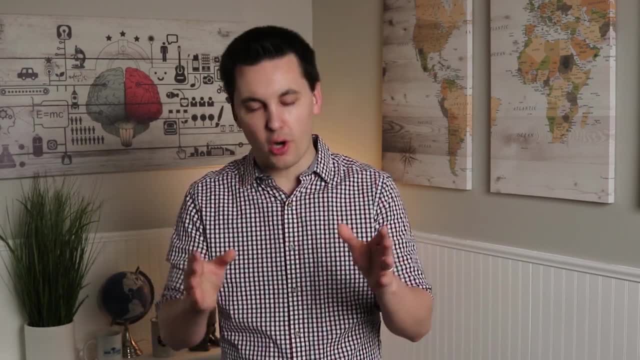 or normal curve. We went in-depth into these curves in our Unit 1, Topic 5 video. I'll quickly review the chart again, but if you need more help with these curves- statistical significance, standard deviations, z-scores and more- go back and watch that video. It has a ton of different. 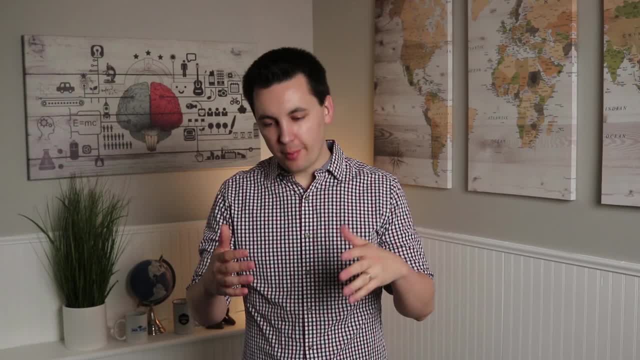 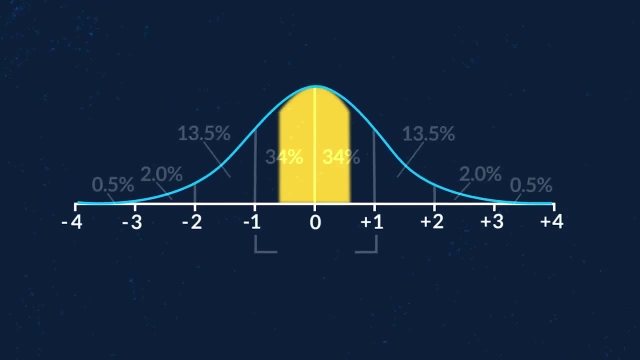 examples and practice problems for all these concepts and much more. An example of a normal curve is the Wechsler Adult Intelligence Scale, a concept from our last video. we can see that, on average, about 68% of the people score within 15 points of 100.